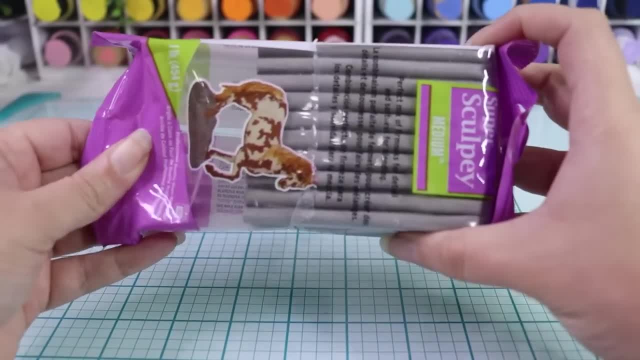 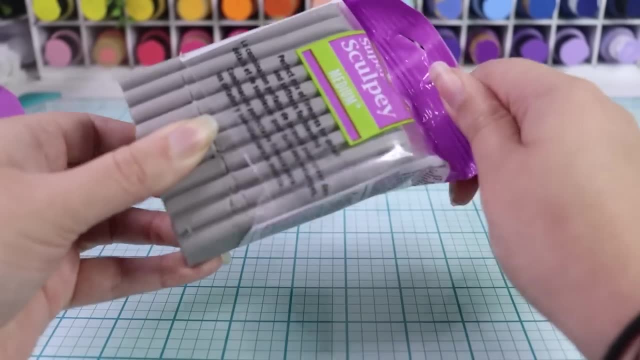 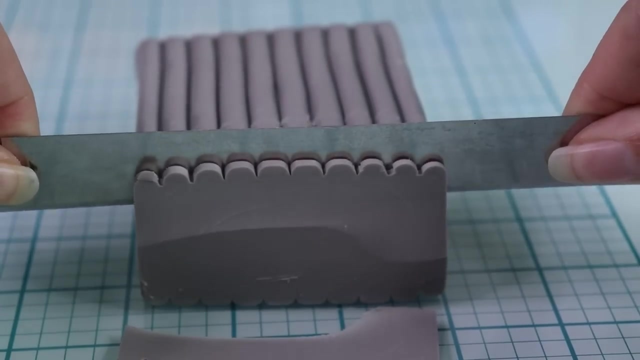 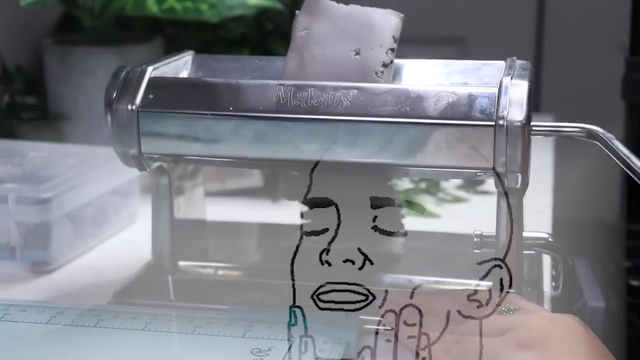 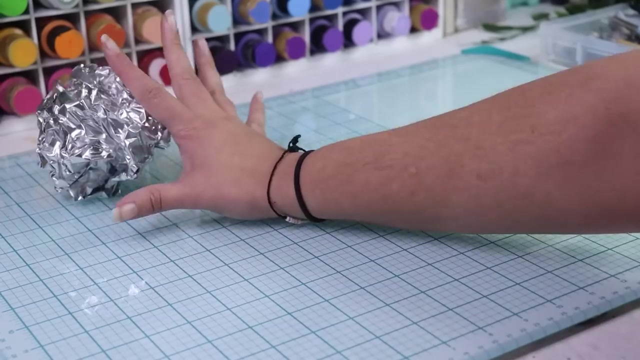 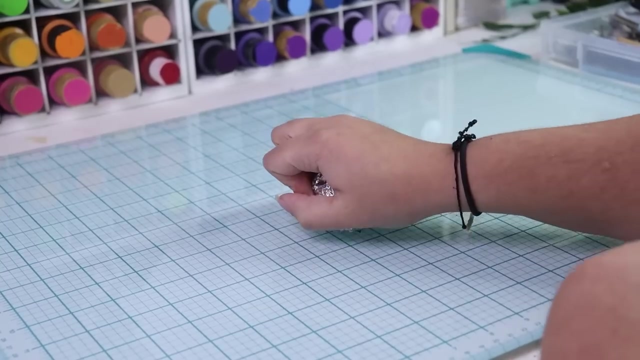 Oh, my god, You are still the problem child. Let go, Let go. Thank you, All right. So first we're grabbing some tin foil, aluminum foil or good old aluminium foil and squishing it into what we're going to call friend shape. 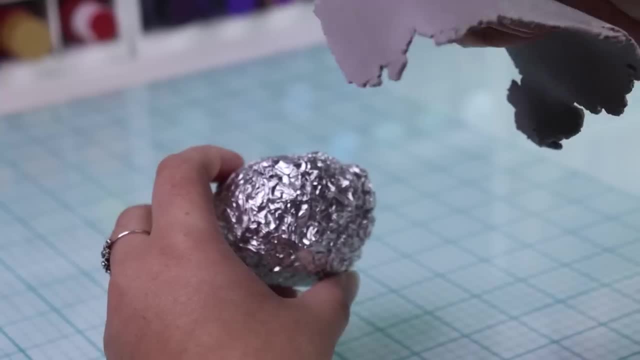 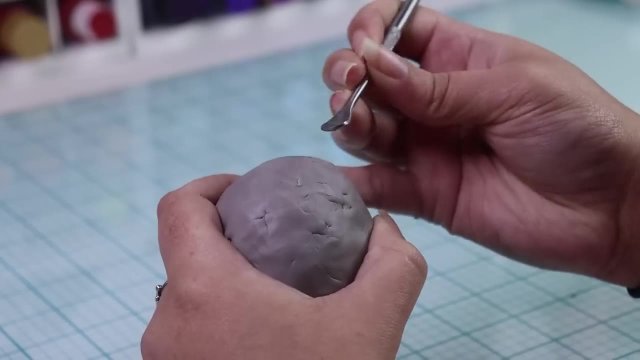 Since the clay is too lazy to sculpt itself today, we'll have to do this the good, old-fashioned way: Covering the foil ball in clay. I'll be starting off with a smooth boulder type of othello, who I've dubbed. 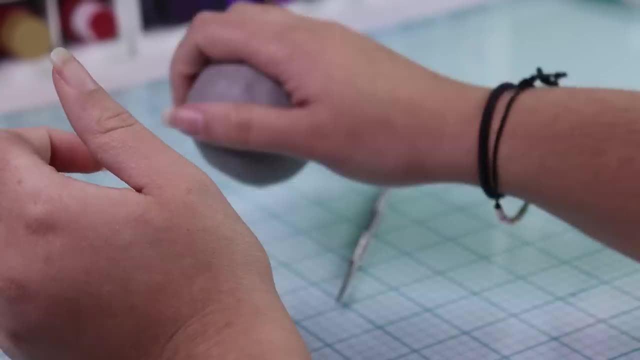 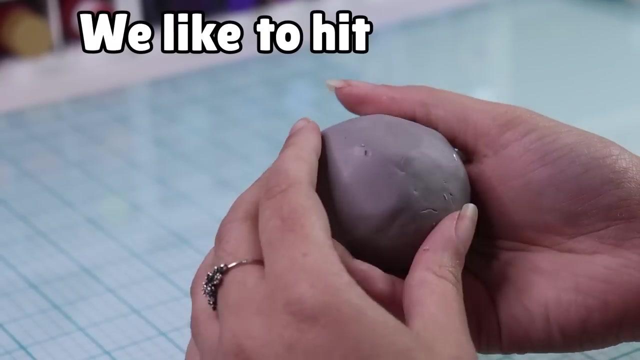 Tinkler Bang to me. As you can see here, I am very scientific about how I add my rock texture, So scientific We like to hit them once and we like to hit them twice and it's a big old ball of clay. 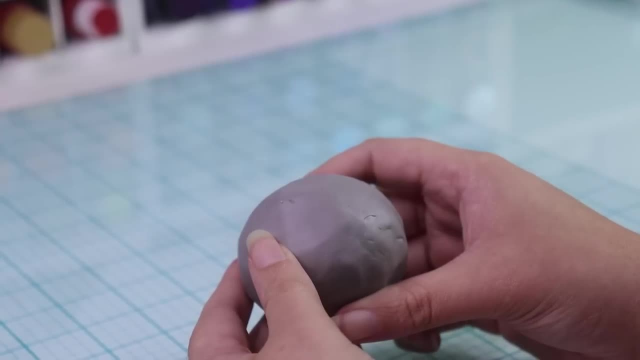 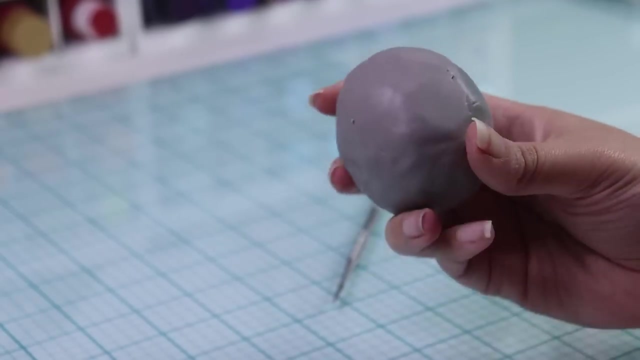 Hey, hey, hey. Big old ball of clay. Big old, You have an ear off, don't you? It's a big old ball of clay Shut up. I bang, skid and sculpt facets into the clay, so it's not just well. 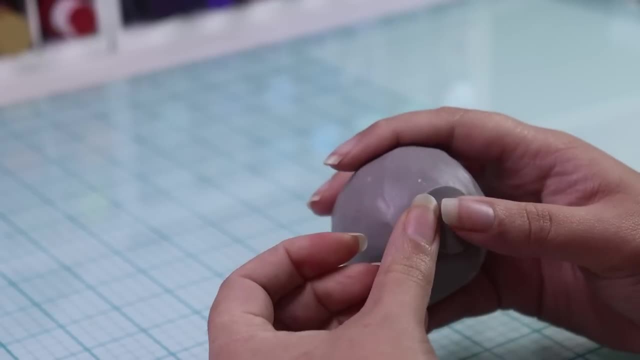 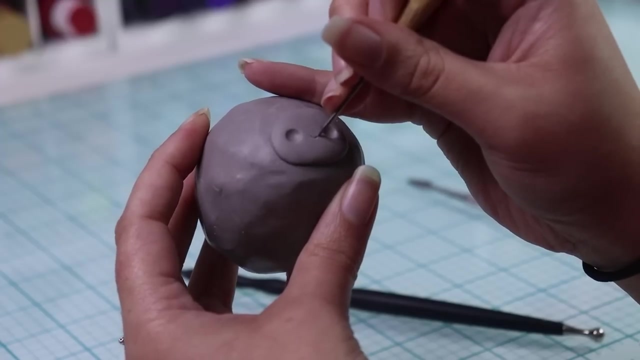 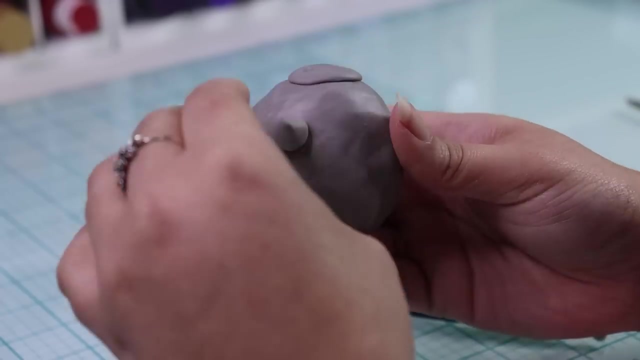 a big old ball of clay. I build up his face a bit since I want to make sure it'll be visible when I add moss later on. Benjamin is a little timid little boulder and is definitely my little spirit buddy. The joy of this idea is rocks come in every type and shape, smooth or jagged. 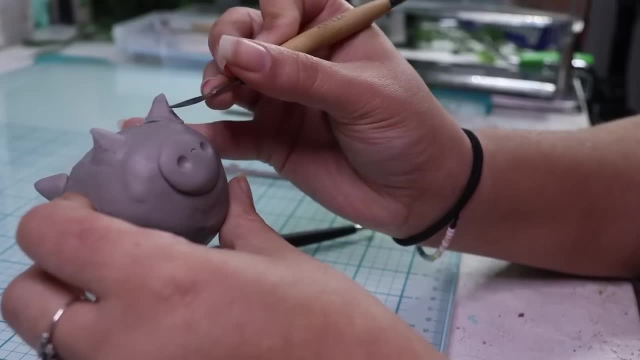 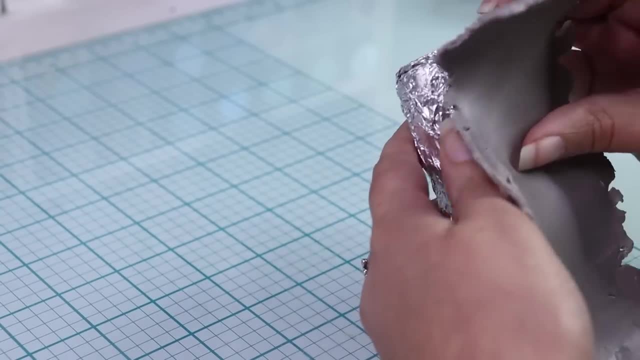 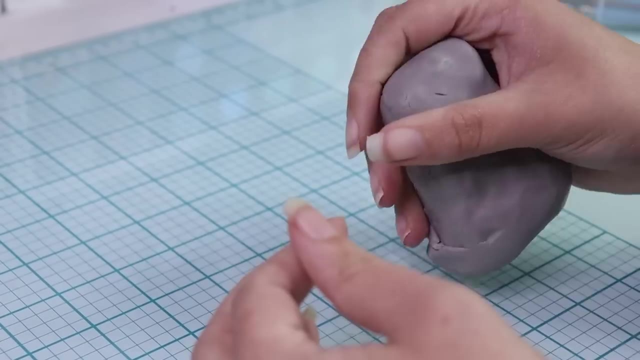 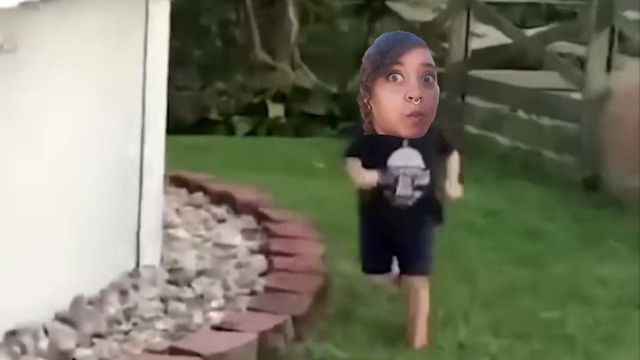 Terrence is up next, and I picture him as a chill go with the flow type of guy who's also down for a little bit of mischief. For him I went for more of a stone slab shape, but I wasn't exactly able to smack him around on my table, so I broke out a knife. Let me see what you have. A knife, No. 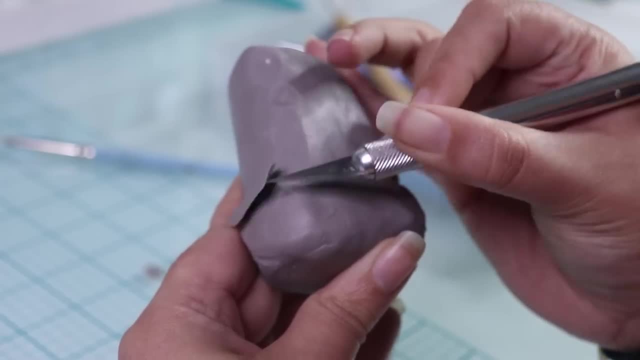 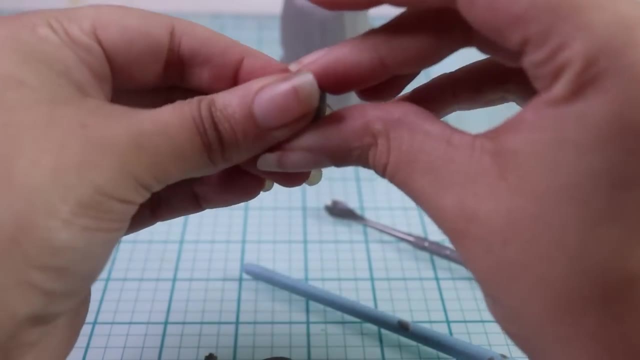 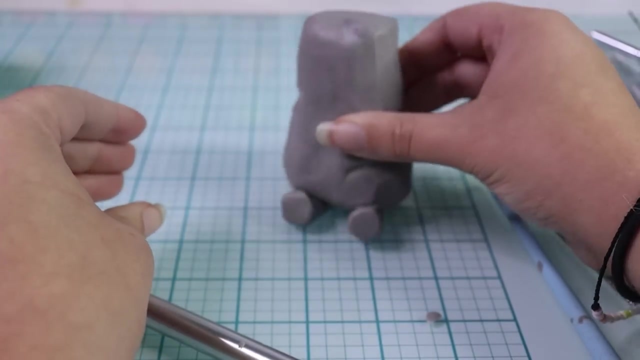 I was able to get some really jagged and clean edges, all with a hint of danger, because this thing was new and sharp. With this big shape, of course, he'd get stubby feet that absolutely would support his weight. no questions asked If anyone who's watching this video suddenly has an urge to. 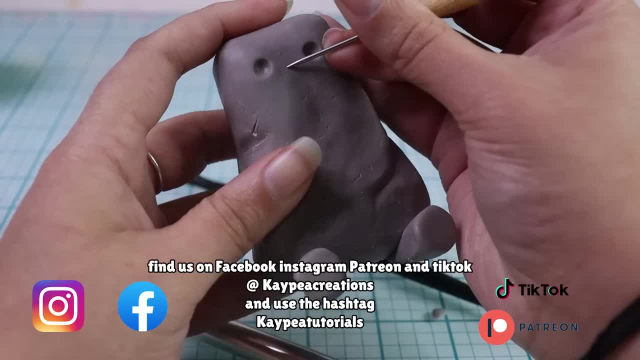 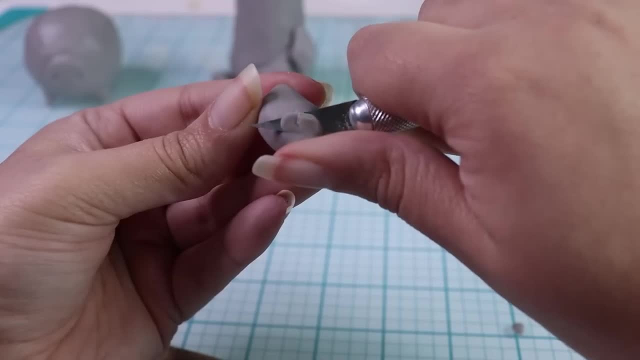 make their own little rock friend. please do it. and then tag me, because I want to see a bunch of little mossy boys that everyone's making, because I think that'd be so cute. He also gets stubby little arms, because there's nothing I love more than making big bodies with disproportionately tiny limbs. I also want to show you a picture of a guy who's a little bit bigger than I am. I also want to show you a picture of a guy who's a little bit bigger than I am. I also want to show you. 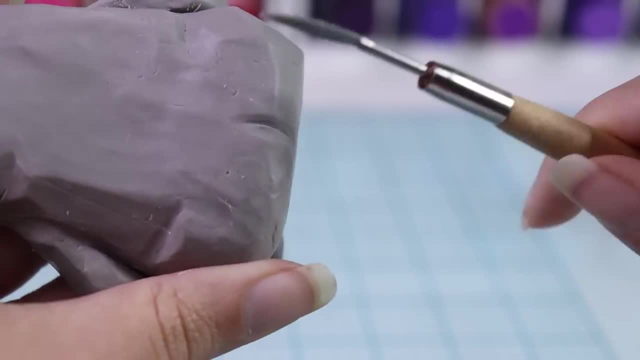 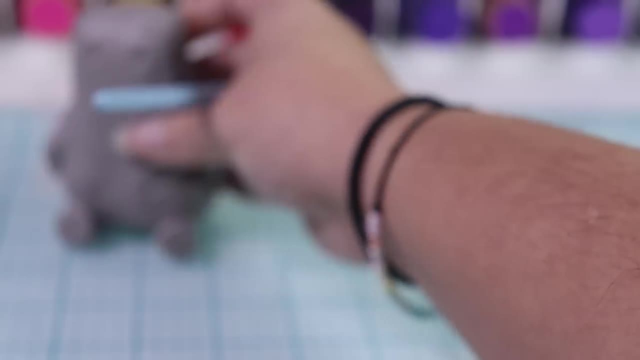 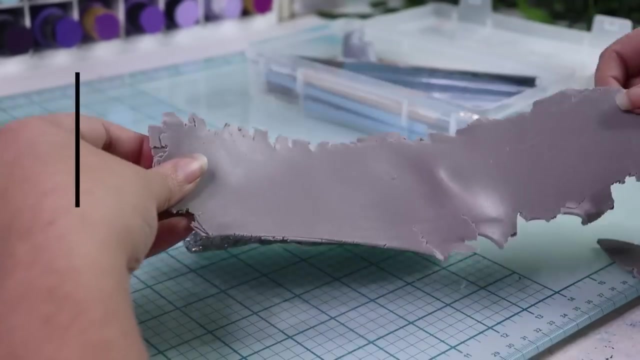 a picture of a guy who's a little bit bigger than I am. I also couldn't resist giving a little rock booty, because I mean, do I even need a reason? rock booty, only a reason. then we have tall boy stanley, the awkward as all heck, but sweet as can be stone pillar, a big boy. 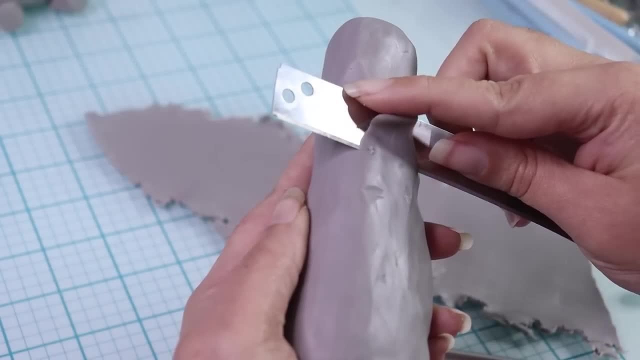 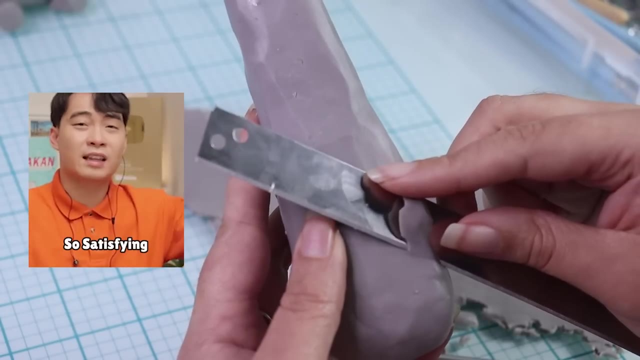 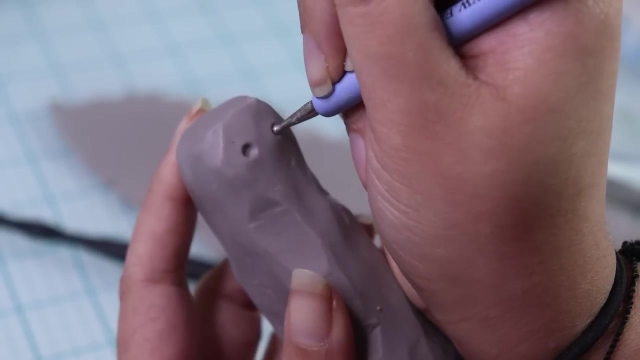 like stanley, also needs a bigger knife to get them sweet rock edges, and I went to town with him- maybe a little carried away, but it was so satisfying so I don't care. he's so derpy, cute, being so tall, with a tiny, itty bitty face. 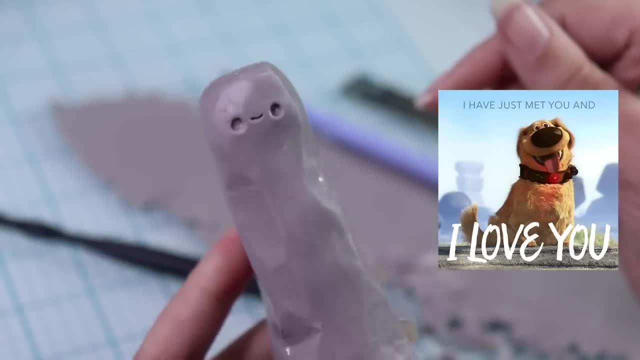 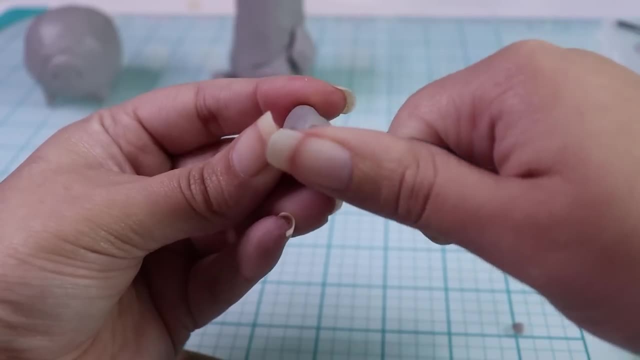 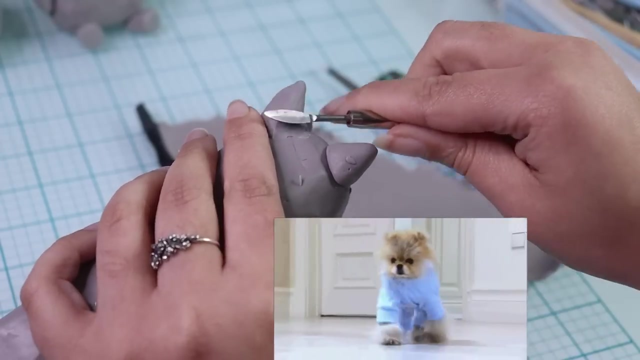 it's giving golden retriever energy. hi there, I have just met you and I love you. remember how I just said: there's nothing I love more than making big bodies with disproportionately tiny limbs. well, I took it to the max with him, to the point that I can only imagine that he just shuffles to get around to a better place. 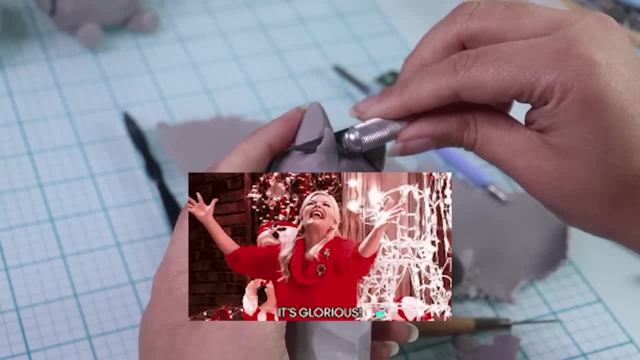 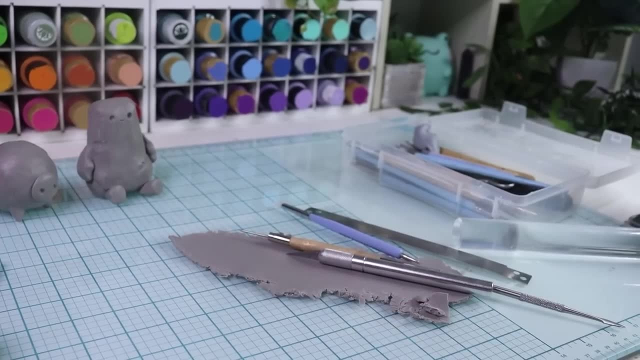 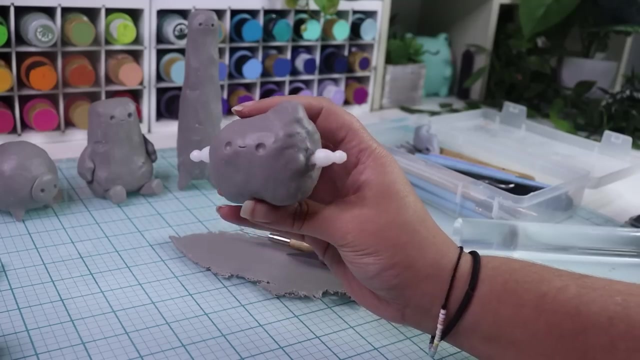 anywhere and that's a glorious image. so we got the boulder stone slab and the pillar. don't forget jerry, jerry. we got jerry back there. jerry's a tumbled rock who got tumbled too much. editor sarah's making her own. this is jerry. show him, show him the back end. jerry got a butt. 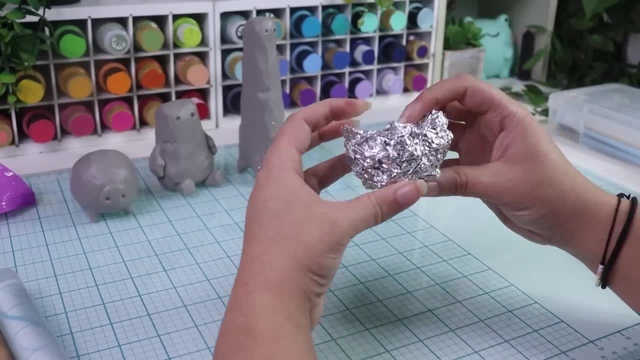 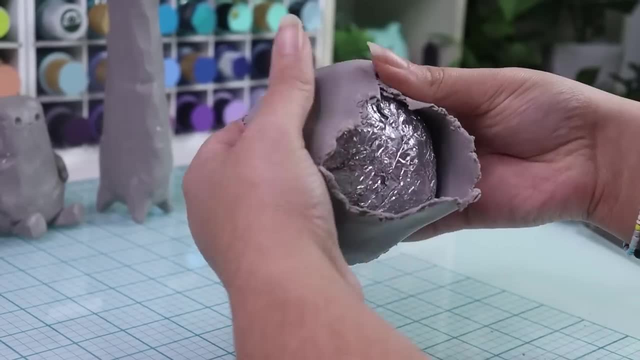 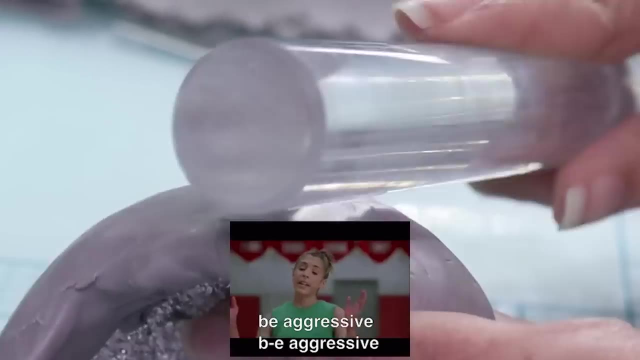 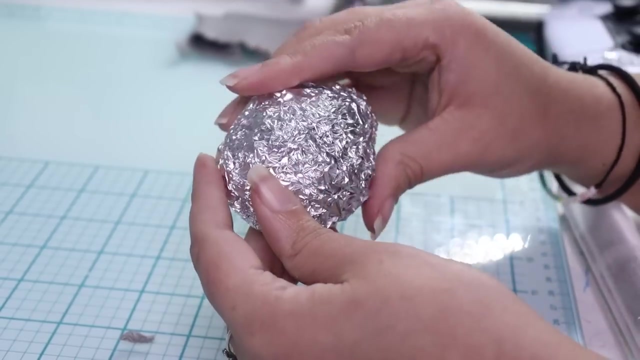 next up is: i'm oblivious and never know what's going on. rock boy kevin, who is also me. i'm not sure what to call his shape. basically he's a planter rock, a rock that has a big cavity where moss now grows like a geode. oh my god, i should make crystal version someday. i used a foil base and clay to. 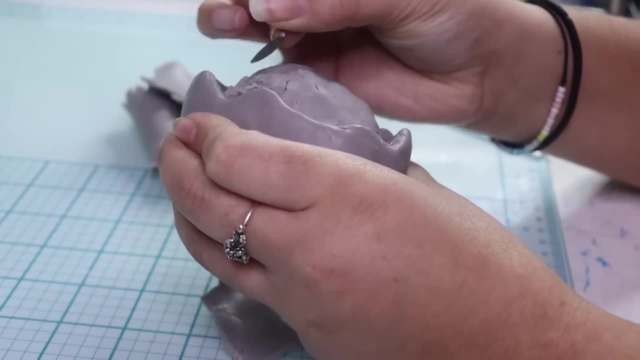 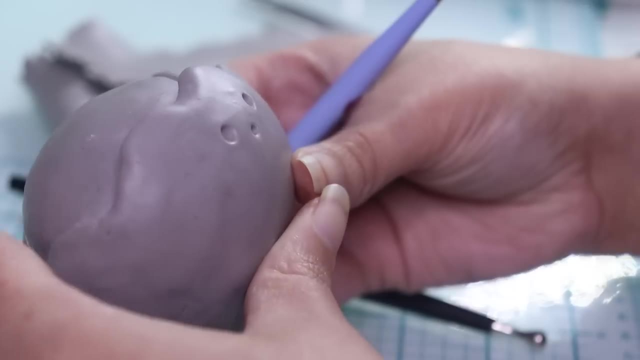 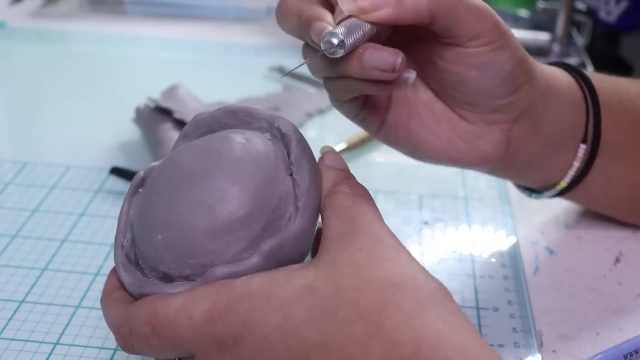 give the impression that a perfect little moss ball is nestled in the center. i gave kevin a dopey expression. we're just saying a lot when it's literally just three dots, but you can't tell me. that's not the vibe you get. kevin is a mix of benjamin's and terence's texture, with some jagged. 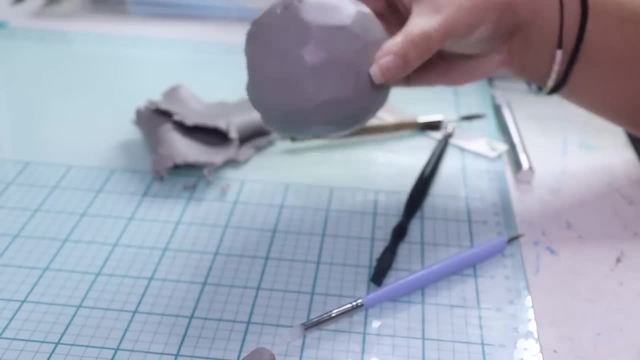 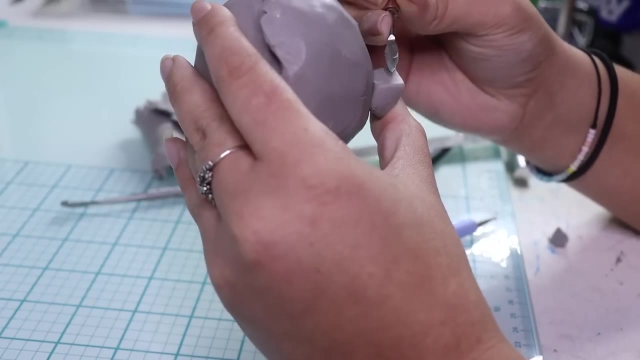 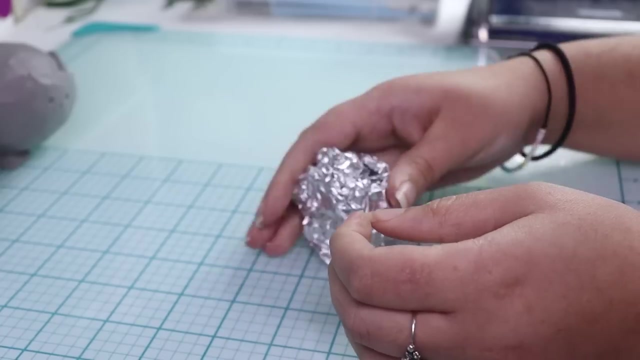 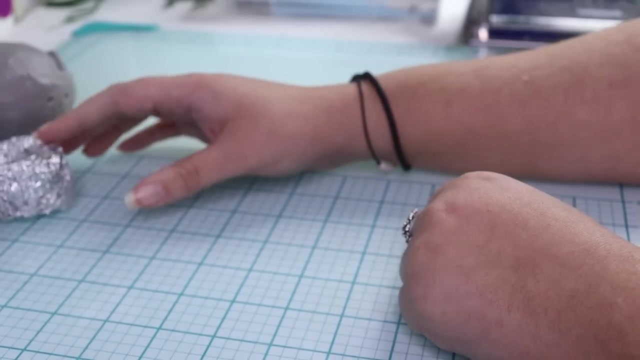 cuts at the top and aggressive smacking at the bottom. you now do i have to tell you what kind of feet he got: stubby, numby ones. i decided the rock squad needed some other friends. so when i was done- procrastinating because once again the clay was not making itself into beautiful art- i made what me and 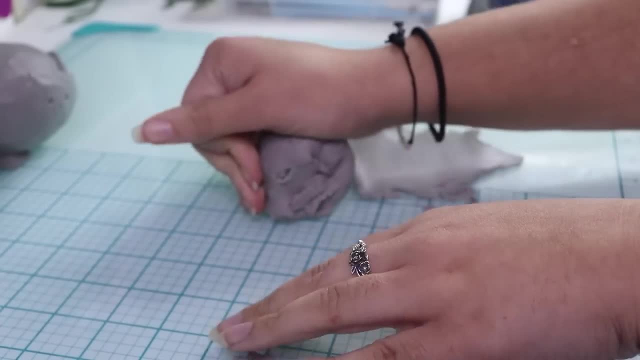 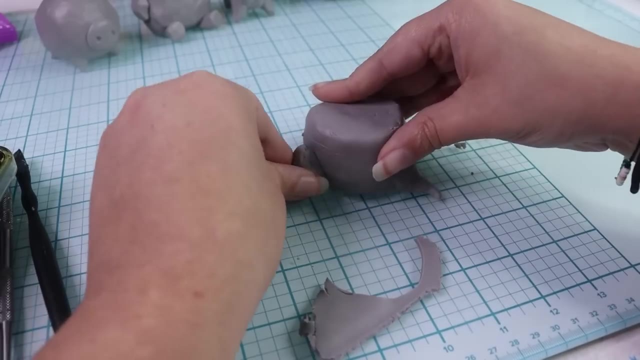 editor sarah, have been calling stump free. now stump free is a hell of a name for a happy go lucky. stump and his best friends would be- you mean, not the most mobile of bunch, but the rest don't mind- just hanging out with him. i enjoyed building up the stylized shape for him. 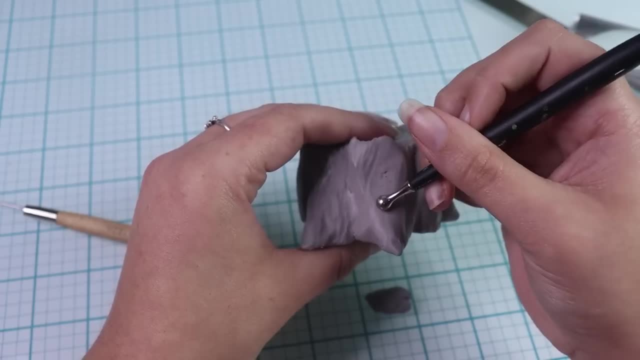 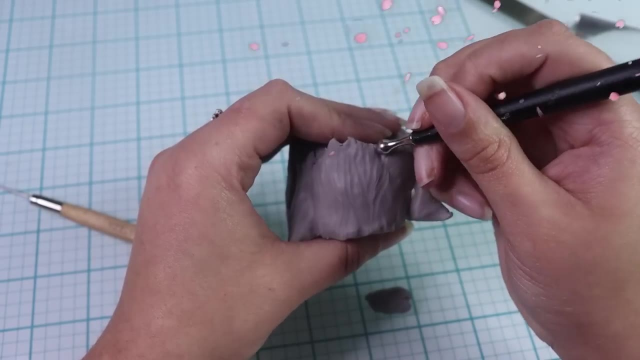 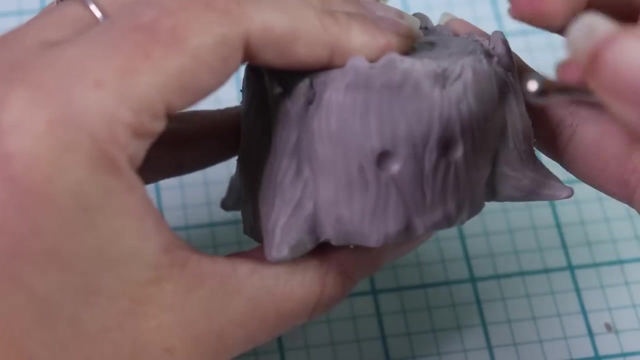 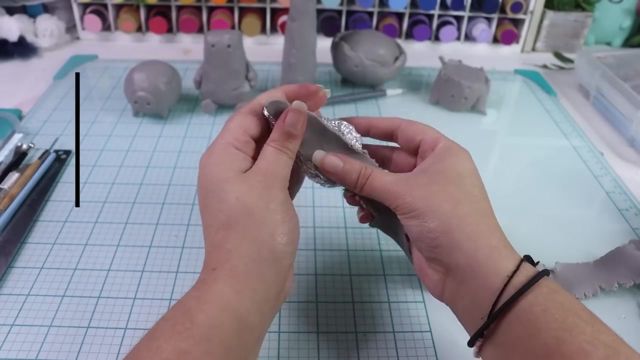 especially the wood texture was just me dragging a dotting tool around willy-nilly, but hey, it looks good and it just gives that studio ghibli whimsical vibe. you, he definitely has. i'm just happy to be here, you, you expression, I just I want to hug him. Lastly, we have the motherly red-capped mushroom, Geraldine. 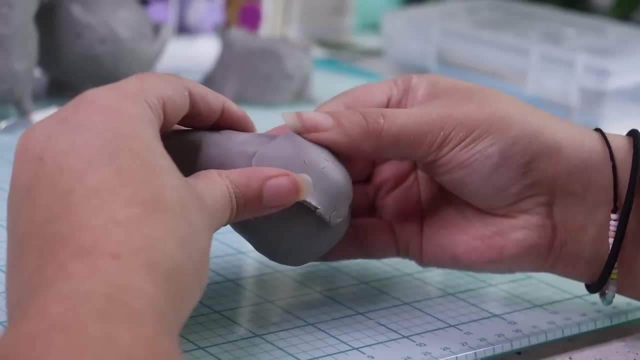 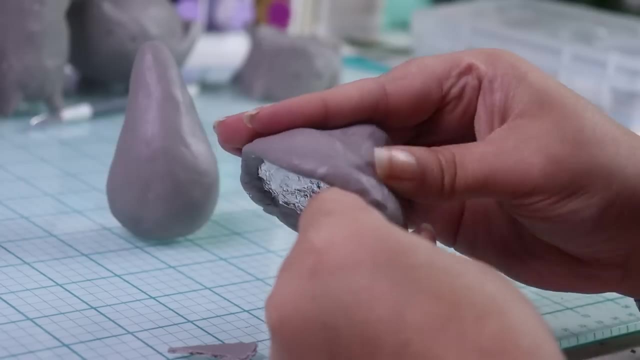 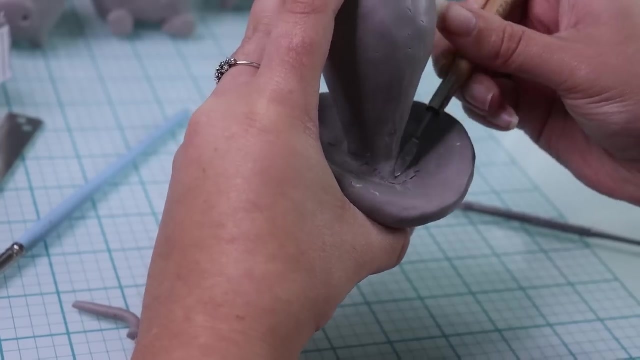 Geraldine is definitely the loving grandma type of the group that everyone wants a hug from, but who also keeps everyone from getting too rambunctious or stuck, Especially Stanley, who keeps forgetting he's tall. I was worried about making her too top-heavy, so I didn't want. 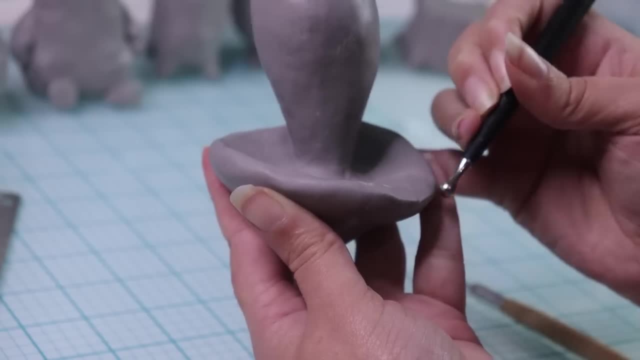 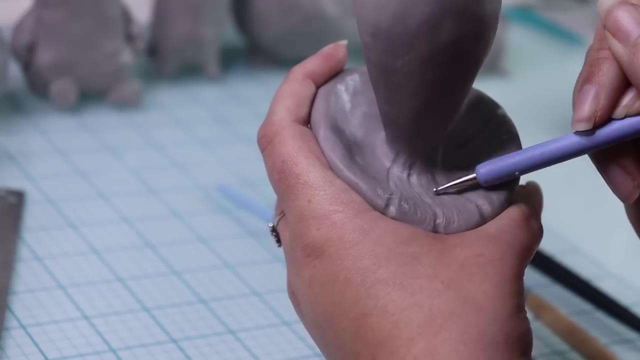 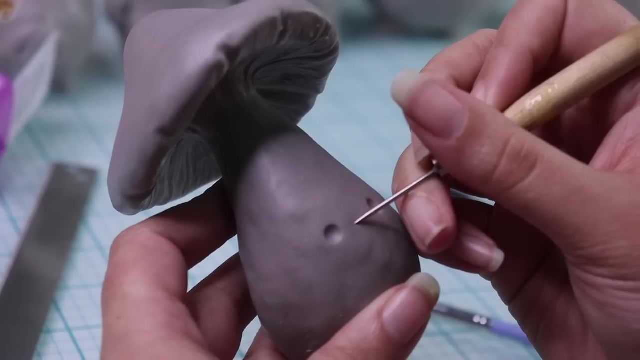 to build up the frill underneath her as much as I wanted, just to help keep her stable, because we were already dangerously close to flop over town. And you know what happens when grandmas fall: I've fallen and I can't get up. She gets a chipper expression since this little fungi is all good. 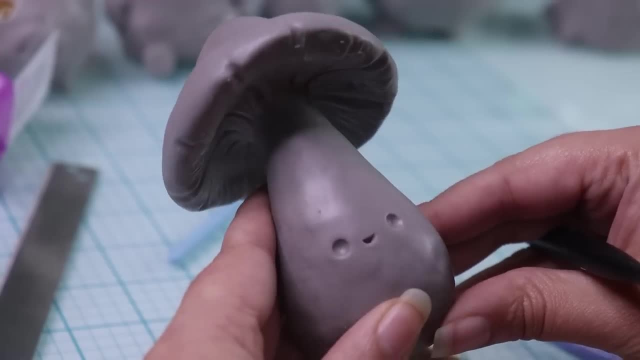 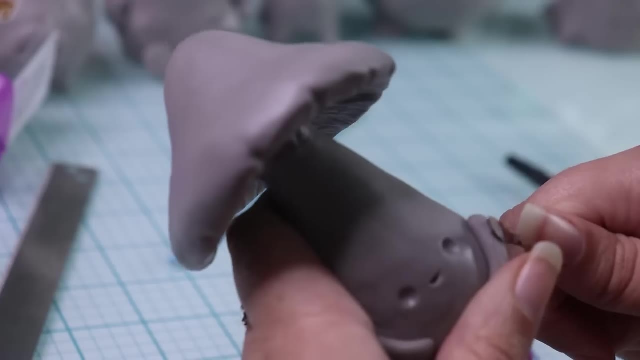 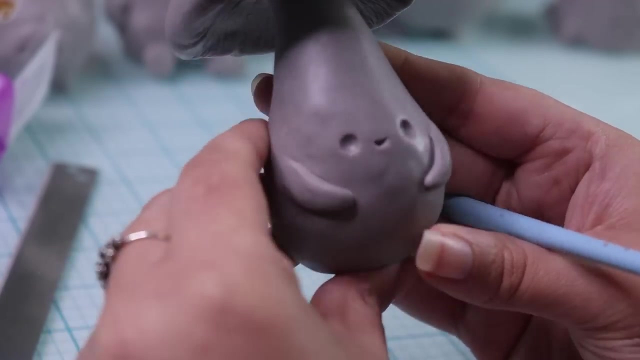 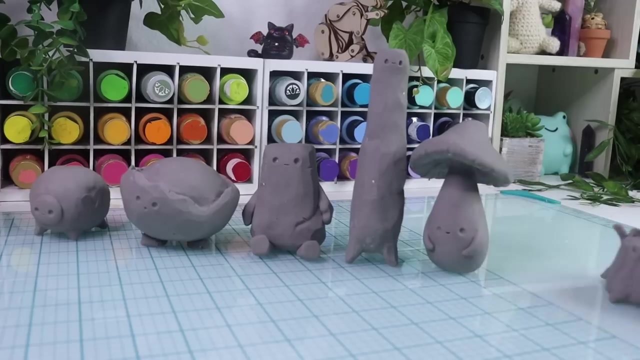 vibes. She had to have little arms because they're bitter to hug you with, but also they're kind of required for that. so she had to, And with her done, it was time for everyone to take a trip in the oven. With all of them baked, it's now time for painting. 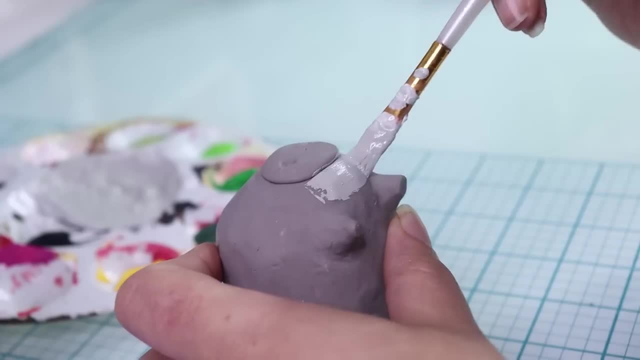 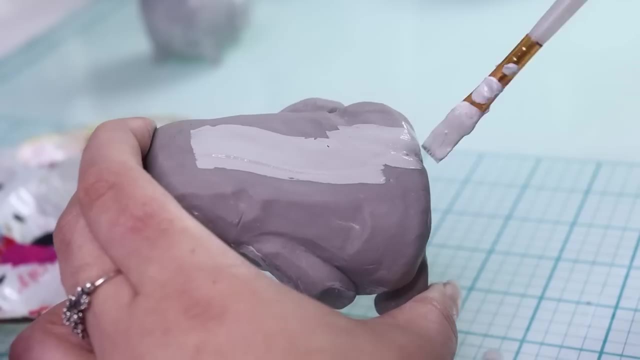 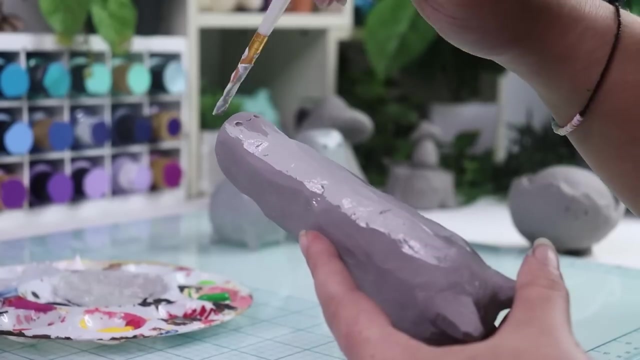 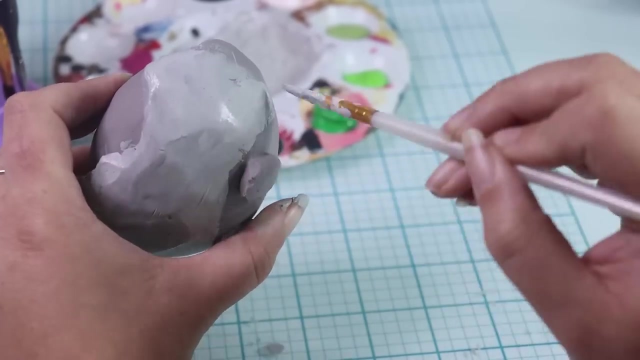 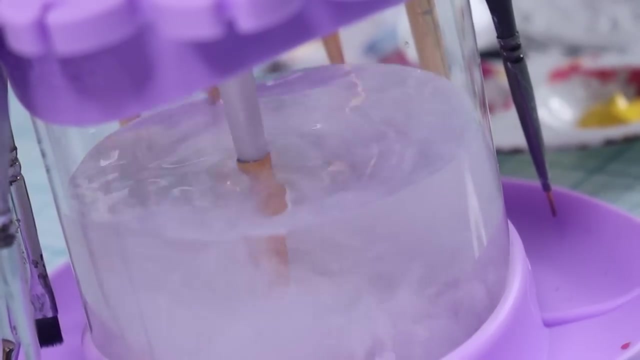 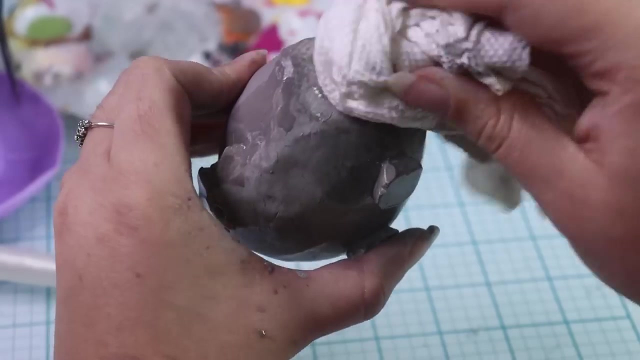 For the painting. I wanted to stick to the Ghibli vibe so I went for light and bright colors. So all the rock friends get a nice bleached rock shade as a base. Then everyone gets a nice dark gravel shade for a wash to really bring out the cracks and divots I sculpted. 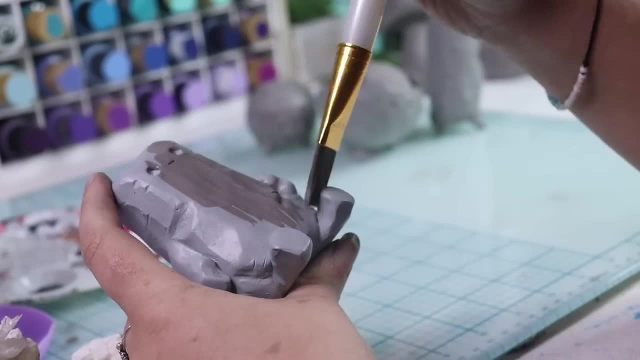 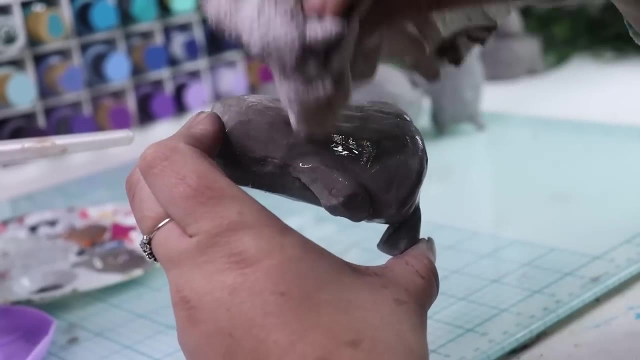 I also dab off the excess with a paper towel. Some really nice woodpeckers, but some still need to be painted. so I start painting answers on all the elements I want. Then I start the many, many layers of highlights, first painting the windows and then painting the. 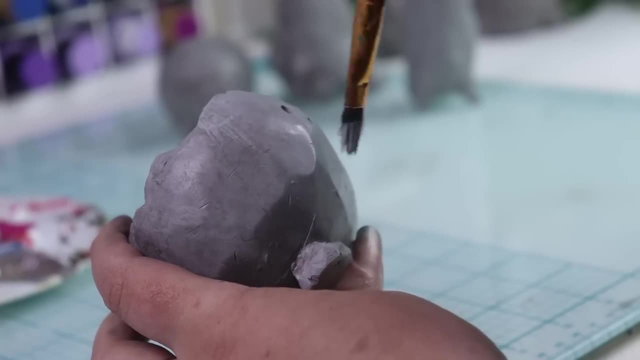 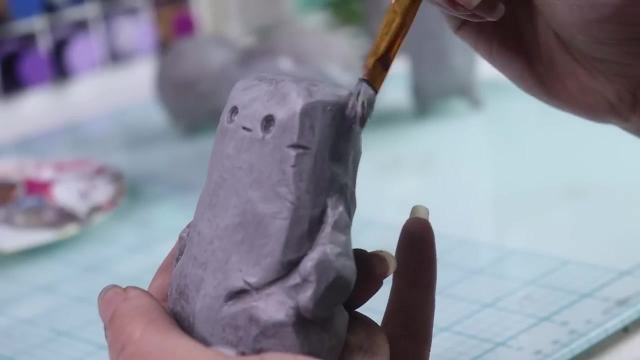 walls. on top of the stuff I wanna make it look like there's something. I then start the many, many layers of highlights, painting all over for general highlights, then using the brightest of my rock shades to just hit the very edges to make them pop. 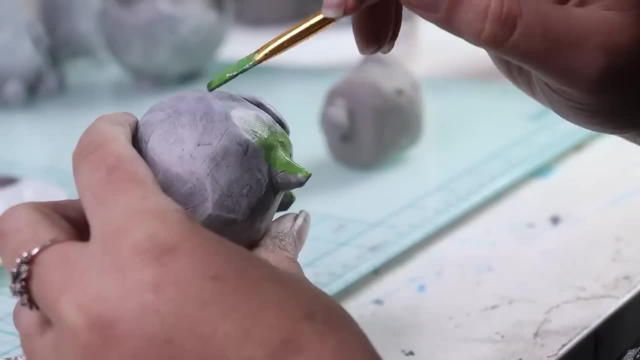 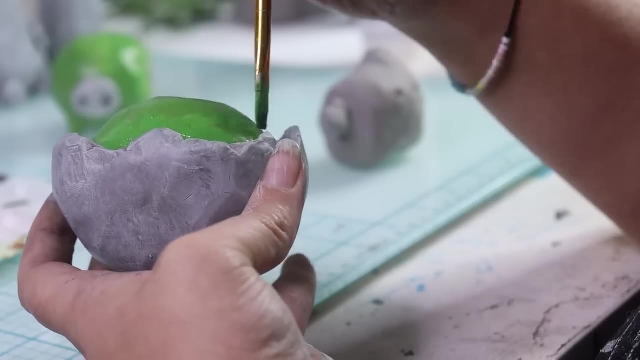 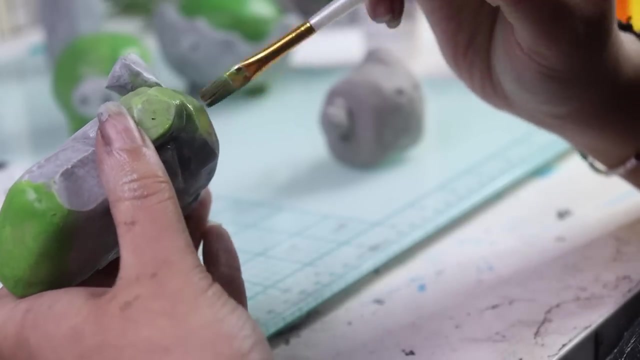 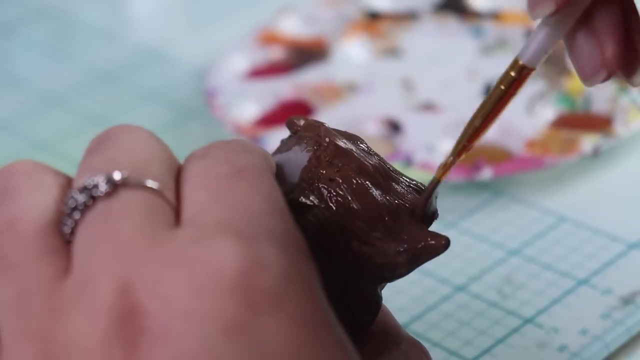 With the rock base done, I paint over where I want all the moss to be with a nice green One part guide, one part. if I miss or mess up, at least there's a green color already underneath. Stumpfree gets a nice dark bark for a base before gradually drybrushing lighter and lighter. 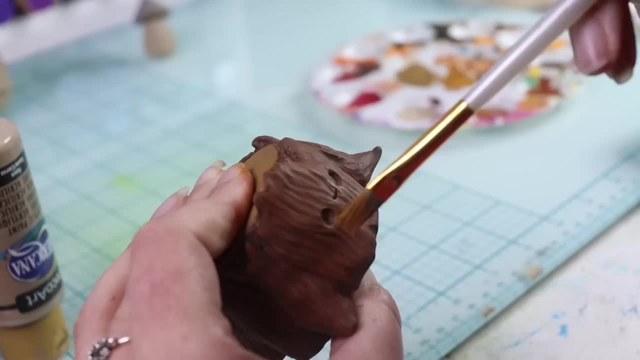 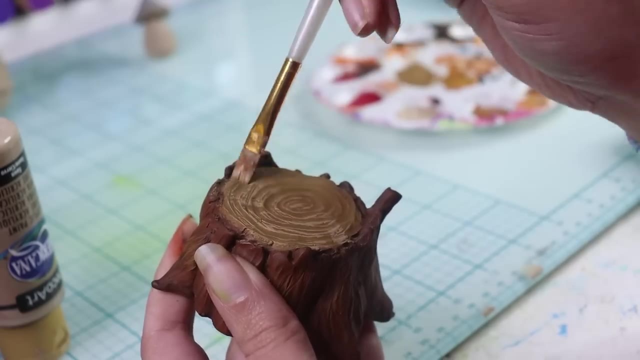 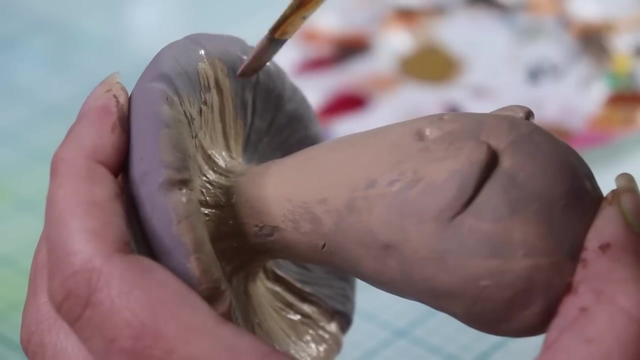 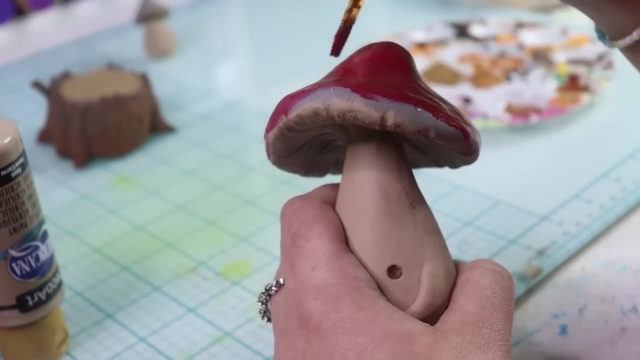 shades of oak, or maybe pine. Either way you look at it, it's a drybrush to make sure all his woodly details pop With practice. from the Mushroom video. I am skilled in the art of mushroom painting, starting with a nice tan for a base, then moving to a deep. don't eat me red for the cap. 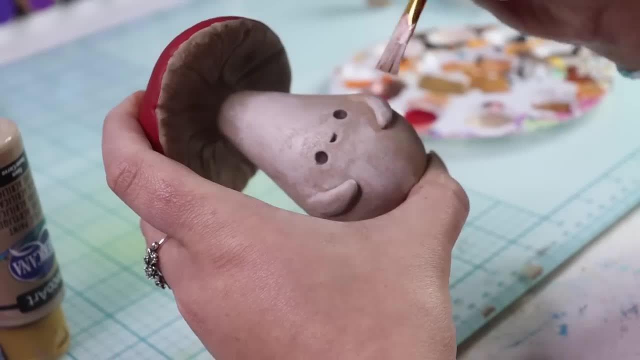 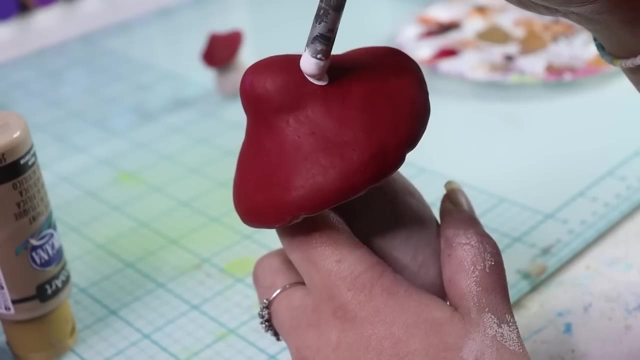 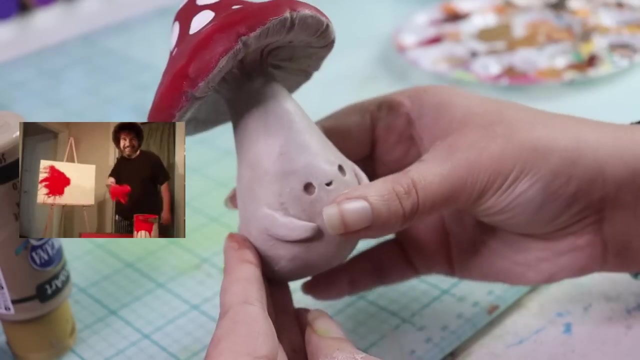 Then drybrushing And a nice bright fungi white. Also can't forget the spots. I absolutely just used the back of my paintbrush. I can't be trusted to paint them and not jerk the brush everywhere. With Geraldine done, it's time to give the boy some moss. 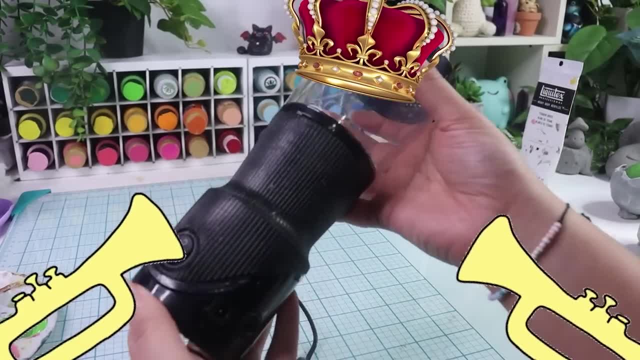 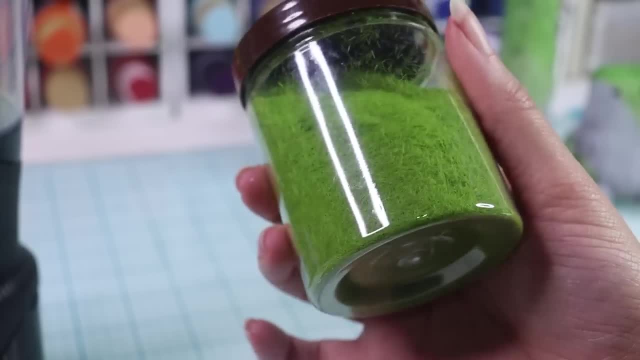 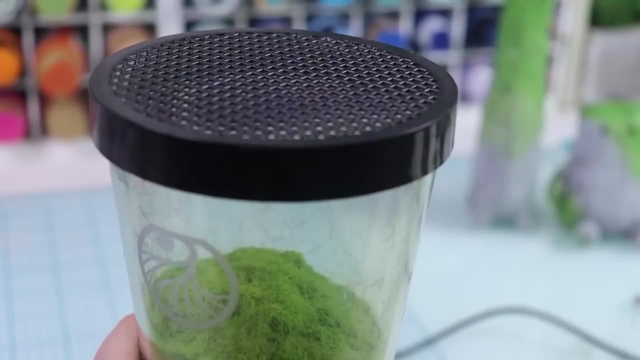 For that I'll be using the king himself, The static king, This magical little mushroom. It's so cute, I love it. It makes grass-like fibers stand straight up, like real plants would, And if you get them small enough they look like fuzzy moss. 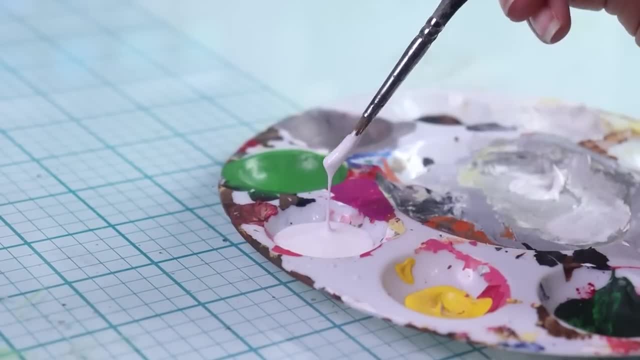 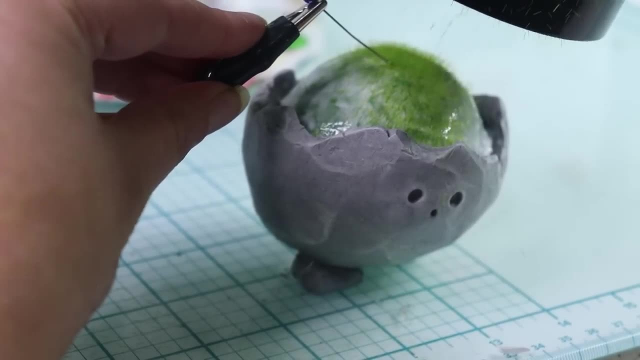 Since I wanted to be accurate about where the moss was, I went and painted on the glue. So rip this, brush You a real one. And once all glued up, you flip the device over and just violently shake it around. It's fun, but god, it gets everywhere. 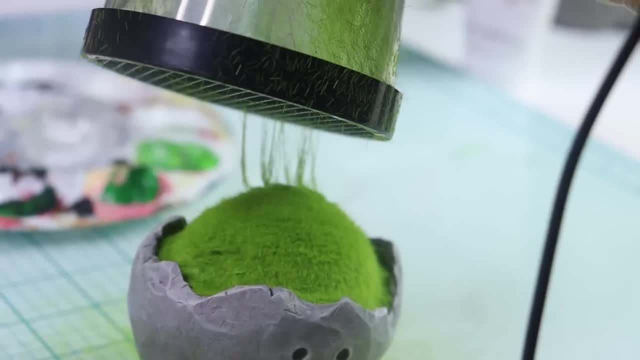 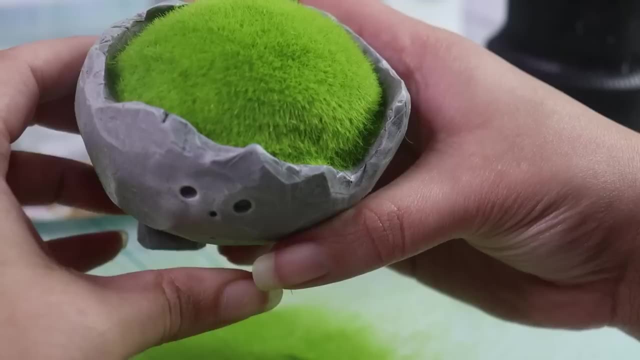 And I just mean everywhere. Camera. Look at the weird strands. It's a monster. This one is not green, Don't touch it, It's not dry. And now it's not dry. I can't touch it, But I wanna touch it. 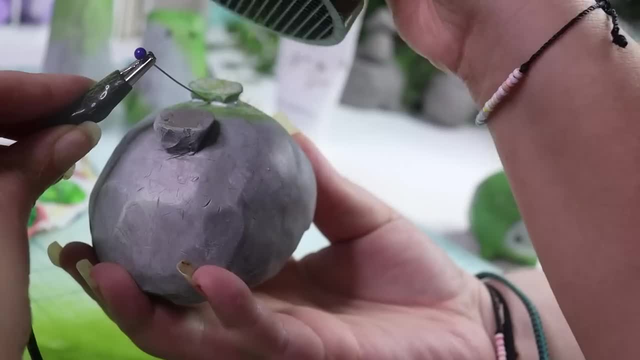 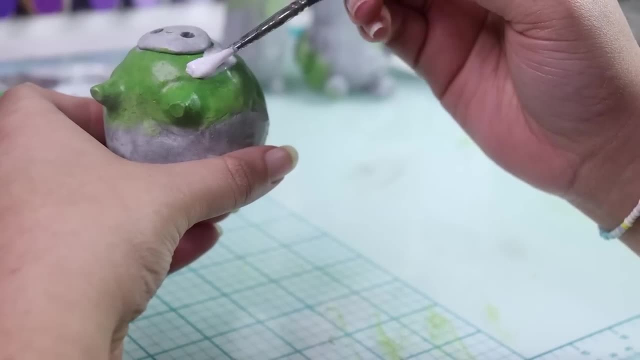 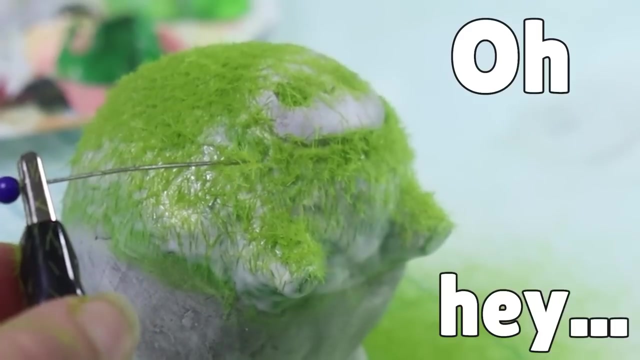 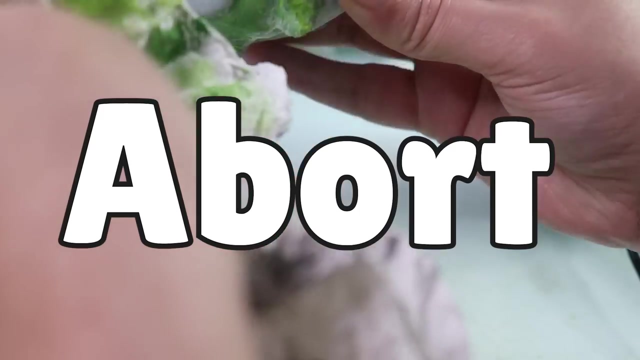 It's so perfect and such a fuSBALL. I then just repeat this step for every green patch I've painted. Good girl, Hm. Oh, Oh, hey, I forgot to turn it on. Oh god damn, Abort, Abort, the mission, Abort. I forgot to turn on the darn thing. 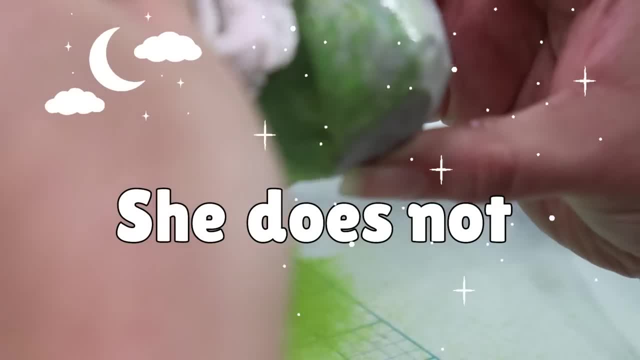 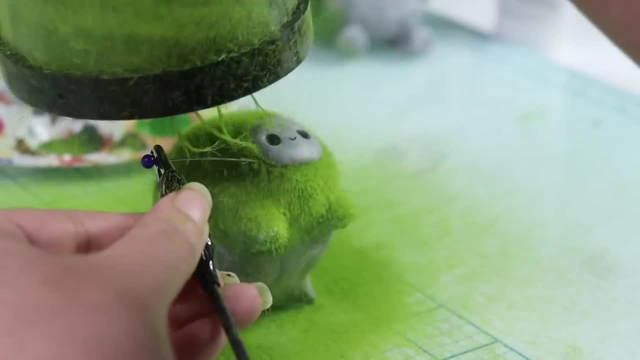 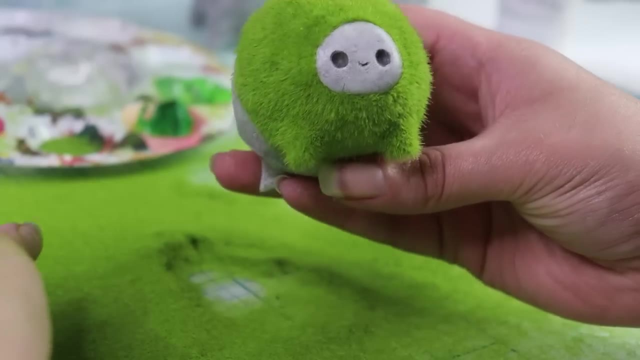 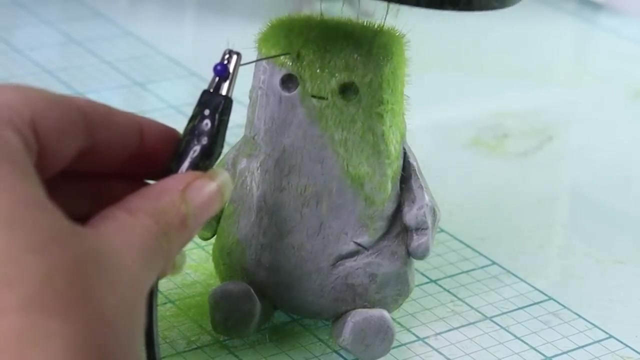 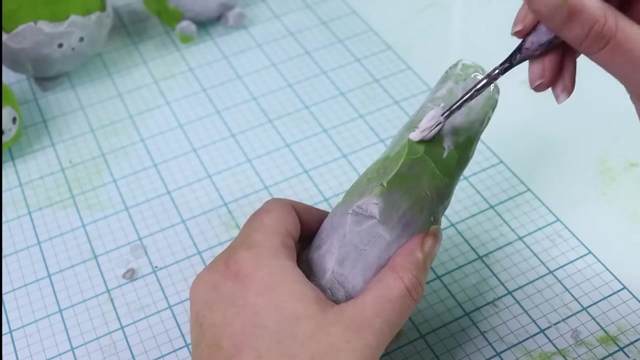 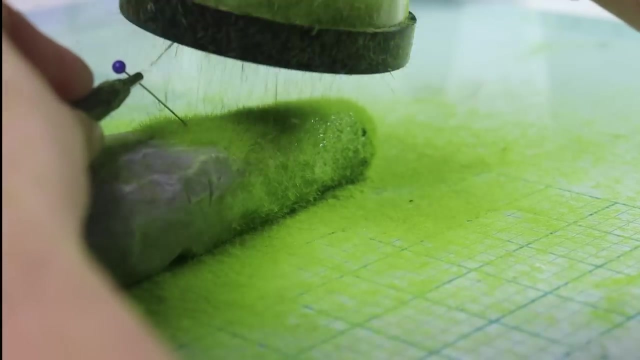 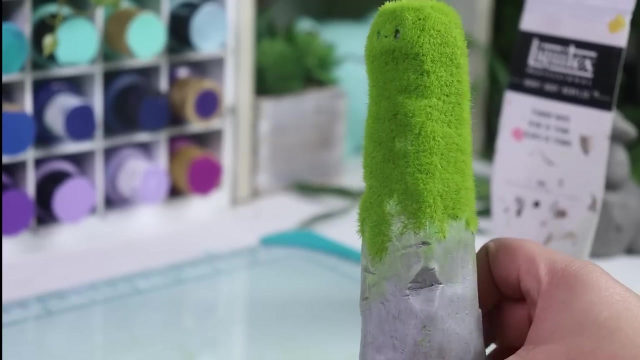 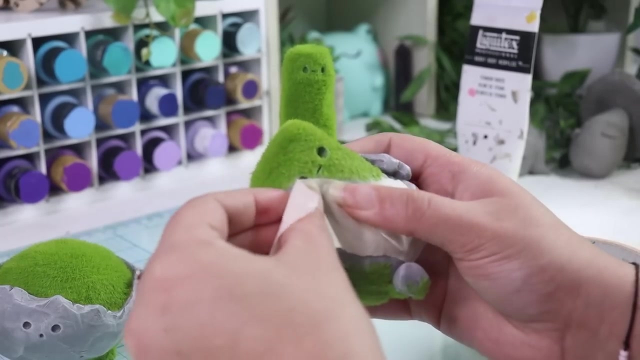 Alright, I think I- When your friend is so dumb, she does not hit the moon. Oh my god, look at you. I'm not worthy. The moss already looks great, but I think I could take it a little further with airbrushing. 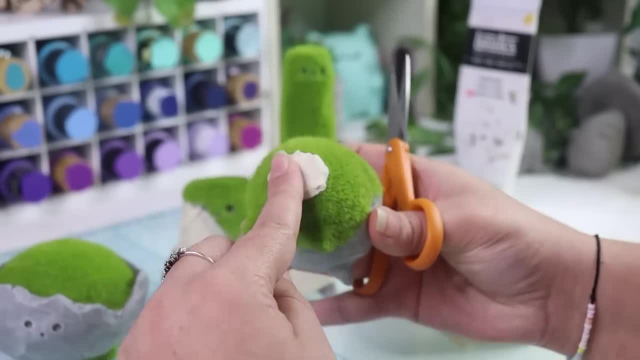 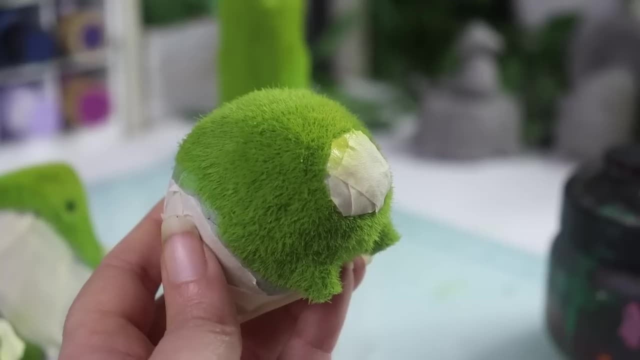 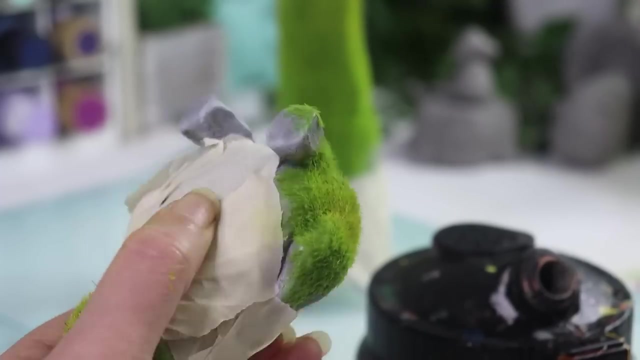 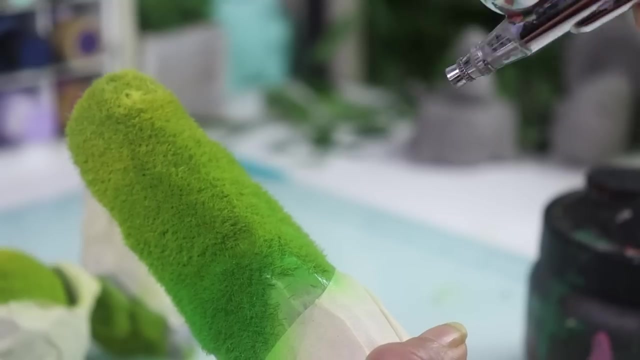 But I gotta make sure to mask off all the stone parts first. I didn't go too crazy, just a highlight and a shadow to give more hues to the moss and make it a bit more vibrant, But I still should have done it in the first place. 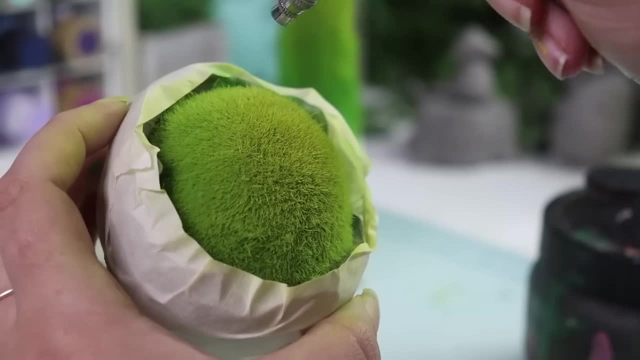 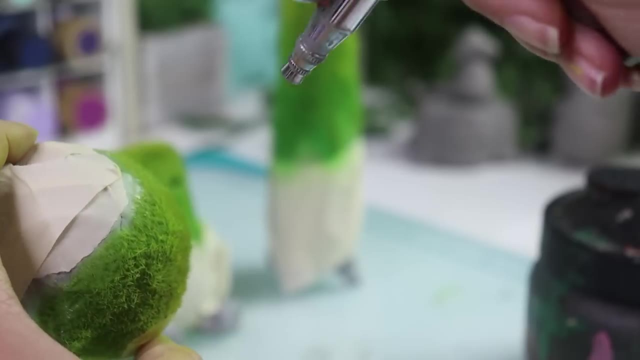 Wait, is that what happened to you? What is he talking about? It was a joke. He was, he was talking about it. He was talking about his own story. He was talking about who he was, why he was in the twenty's, and then he was in his twenty's. 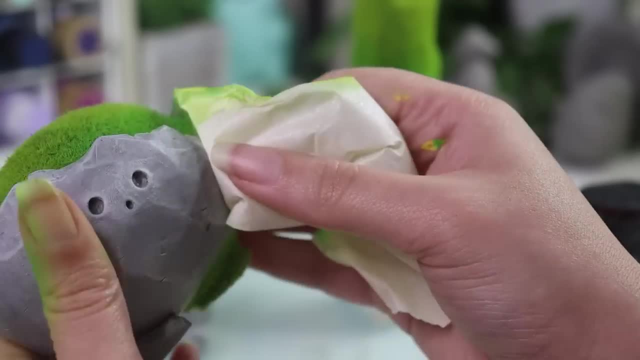 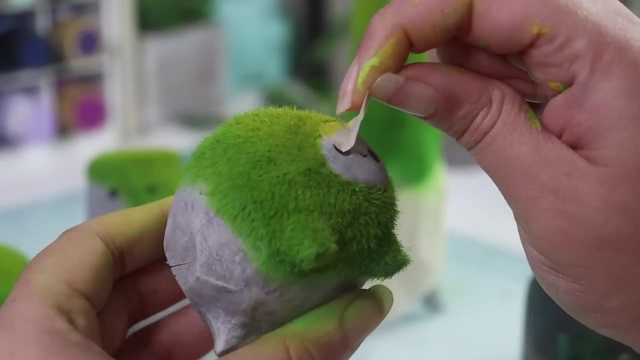 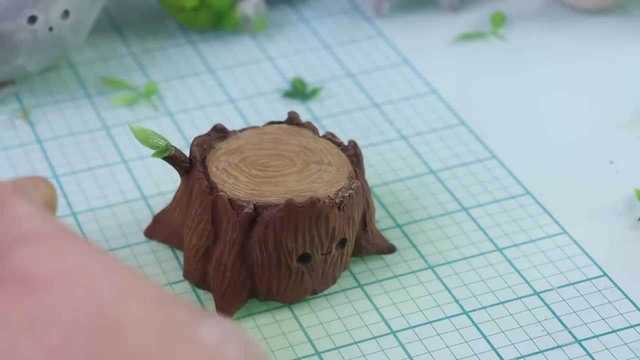 Oh, I really want to know, But he doesn't want to hear what I'm talking about. But he has a lens and he doesn't think that it's important, You don't? You don't? The last step was to just add a bit more greenery, giving everyone their own little seedling. 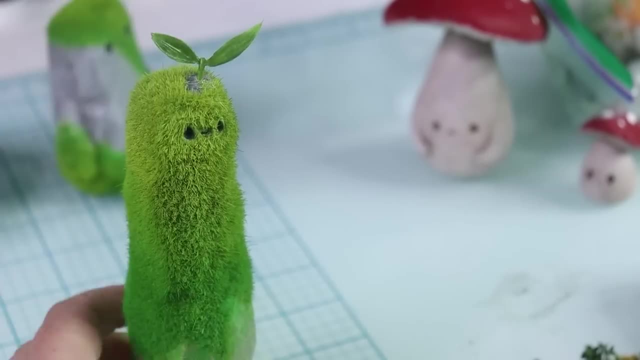 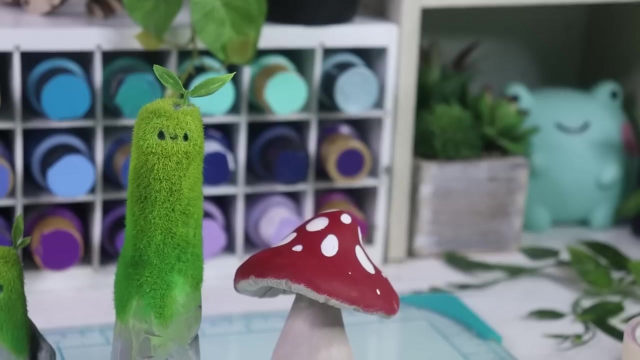 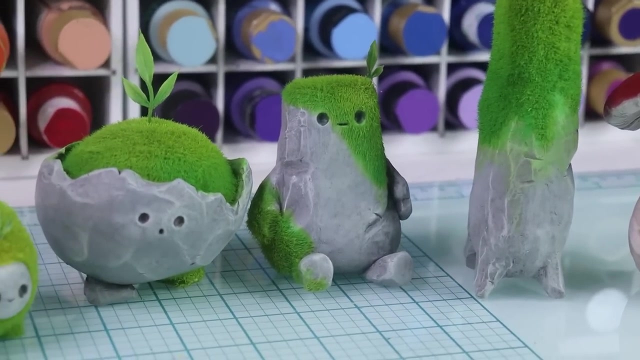 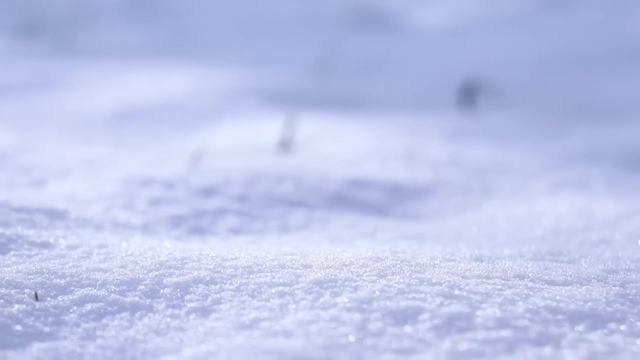 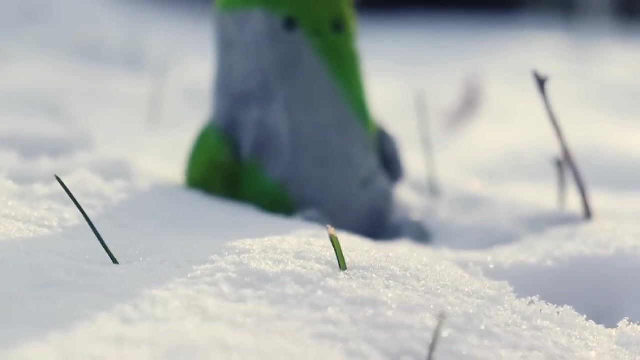 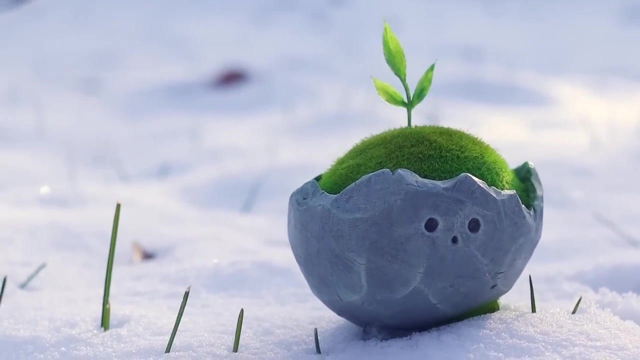 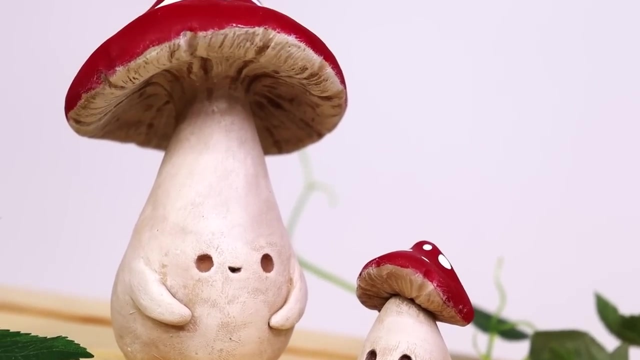 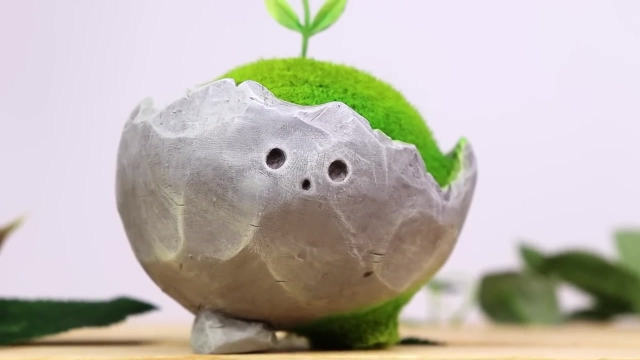 plant to take care of And, with that, the nature. amigos are done and we can take a look at the final adorable montage. Thank you so much for watching and I'll see you in the next video. Bye, Bye, Bye.